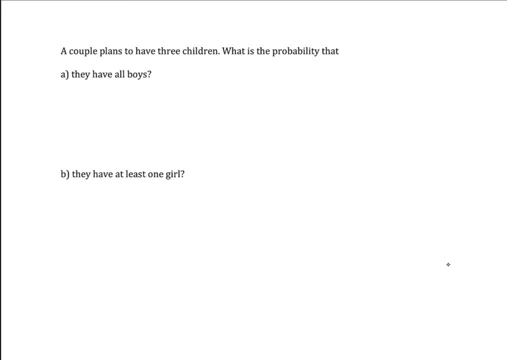 and the second child is a boy and the third child is a boy. So all of those ands joining our events together tell us to multiply events. But before we go and multiply events, we have to make sure we're dealing with independent events or dependent events, So we know if we need to. 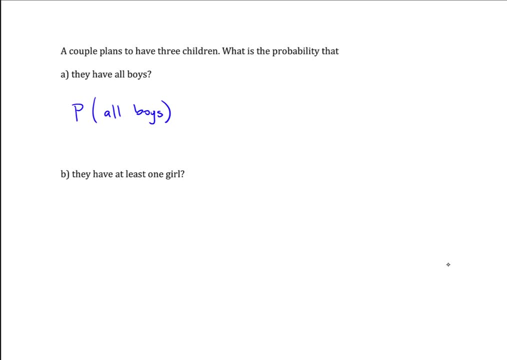 decrease our probabilities from one stage to the next. Here we have. I think the only thing we can really do is assume independence, even though we don't have a large population And, honestly, even though this is one couple which you could actually think that there 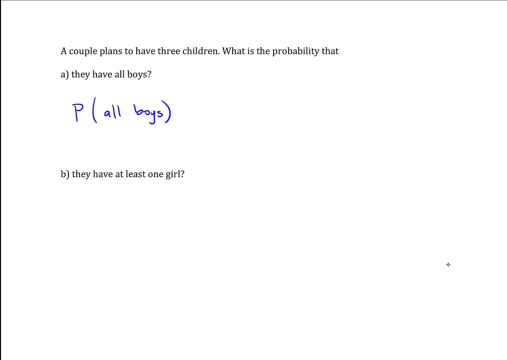 might be some biological component which says that each couple is could be more likely to have more boys than girls. But let's keep things simple and probability and statistics. Let's just assume the probability of having a boy is 50% And the probability of having a girl is. 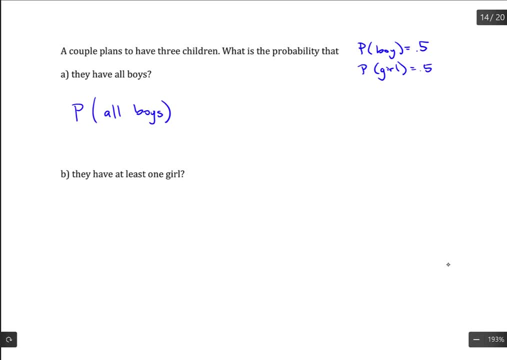 also 50%, So we'll keep it simple like that, All right. so the probability of all boys: So 50% is the probability that the first child is a boy and 50 is the probability that the second child is a boy and 50 is the probability of the third child. so, assuming independence, it's 0.5 to the. 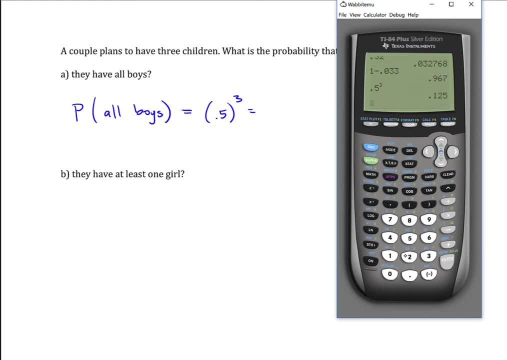 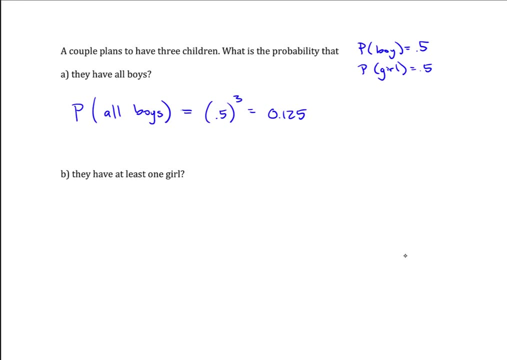 third power, which would be 0.125. what's the probability? they have at least one girl, so at least one girl. there's different ways that you could petition, potentially, think about this. so one way that i have students trying this problem is to do something like: all right, well. 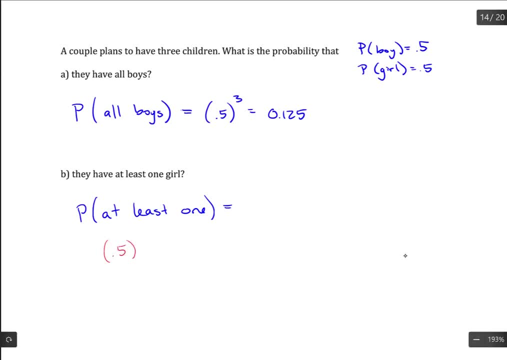 the probability of a girl is 0.5, probability of a boy is 0.5 and the probability of a girl another boy is 0.5. so i have one girl here and then two boys. so that's at least one girl, so that